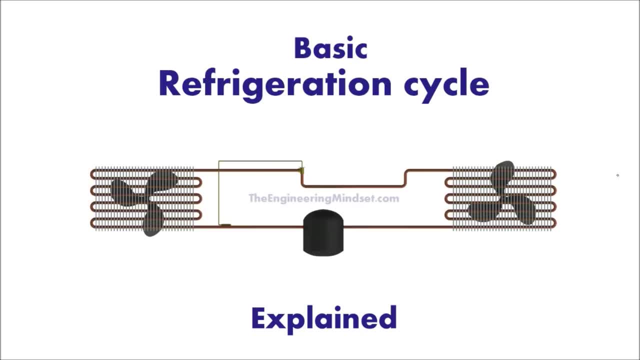 area, from the area, from the room, and then we need to dump it somewhere else. So to do this, we send the refrigerant around And the four components will help that: pick up the heat and dump it. What these four components will do is change the temperature and the pressure of the refrigerant, and that is how 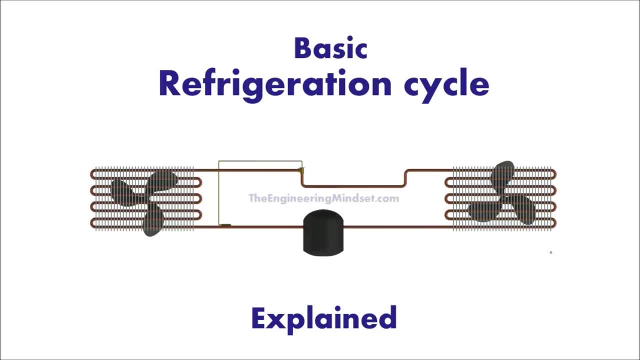 the cooling and heating is produced. So the four main components we've got in the refrigeration system- and these are essential. it has to be in every system for it to work. The first component is the compressor And that looks like that And a real life compressor will look a bit like this one. You see that on the back of 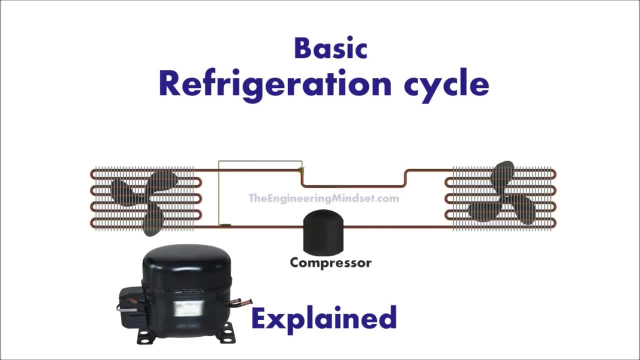 fridges or if you've had the chance to look inside the split AC unit, that would be one of them. I'll leave that for a minute. The second component is the condenser- This unit here That's usually found outside the building. 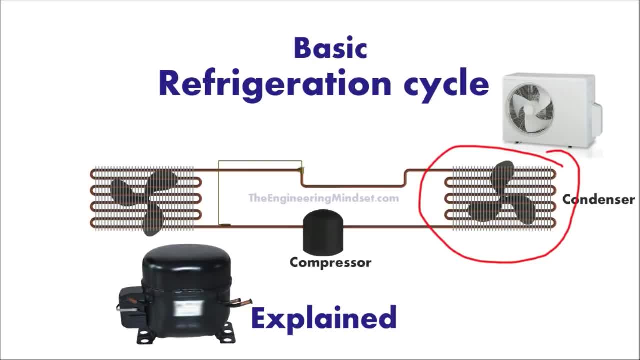 It's mounted on the wall. You know it'll look a bit like this in the real world. And then the third component we'll go to is the expansion valve, And that is this thin tube with this bowl and this valve here with the pipes in between. A real life example. 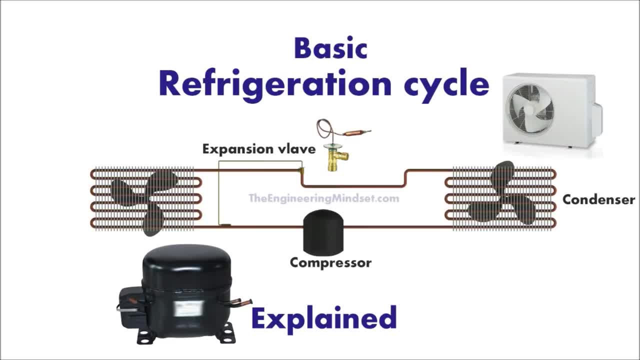 of that will look something like this. one Final component- Final component in the refrigeration cycle is the evaporator. This unit here looks a lot like the condenser in this example, but it won't look so much in the real world most of the time. 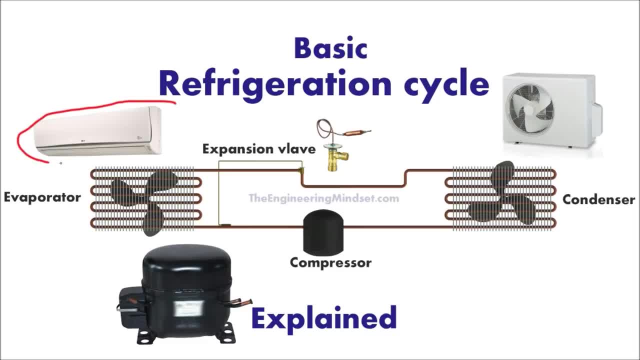 And we've got an example of what one of those will look like. You've probably all seen these before mounting the walls inside the room, and this is where the cool air, cold air, comes from, And it's also which takes the heat away. 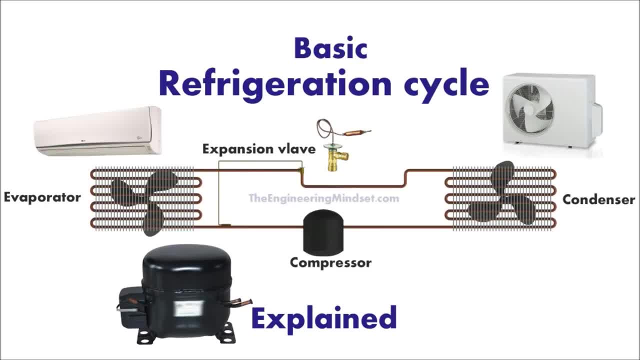 There are four main stages in the refrigeration cycle where the pressure and the temperature change And these all occur within these four components. The first stage, in fact, let me just clear some of these off make some room there. So the first stage: this happens at the compressor And what happens is the refrigerant enters. 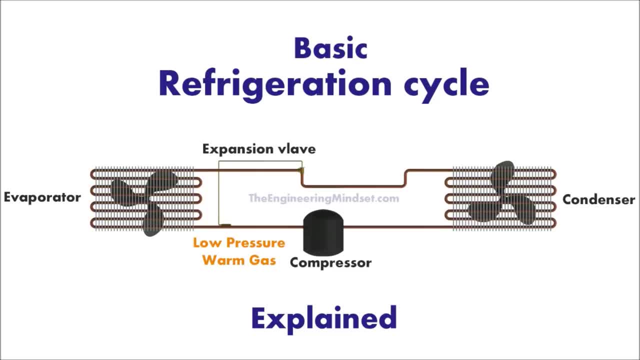 the compressor. It leaves as a low pressure warm gas After compression. it leaves as a high pressure hot gas, And I'll just draw those on there as well. Oh, that one. Okay, There's the high pressure coming out of the compressor. 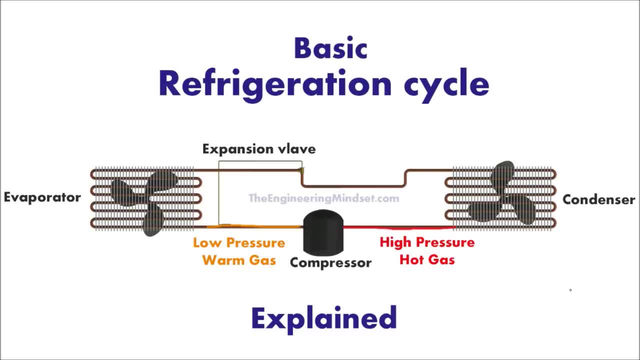 So for the compressor, when you compress a fluid, the volume decreases and all the molecules that are in there get pushed closer together. The quantity is still the same, It's just more compact now compressed, Okay. When this happens, it causes the temperature to increase as well as the pressure. 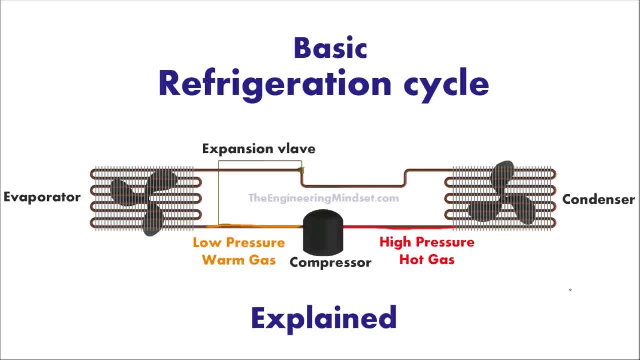 And, as I already mentioned, for the refrigeration cycle to work, you must be able to dump heat somewhere. The air in this somewhere else needs to be cooler than the surface temperature of the pipe on the condenser. If these two- if the surface temperature of the pipe and the air in the around the condenser- 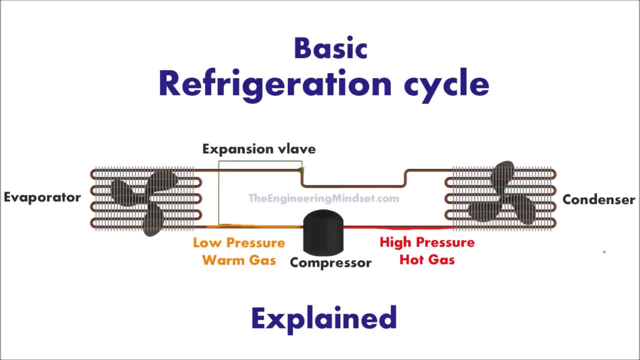 if they were the same temperature, you wouldn't be able to dump any heat, So you wouldn't be able to cool the room down. So to ensure the pipe is hotter than the air around it, the refrigerant is compressed to a higher pressure, which obviously increases its temperature. 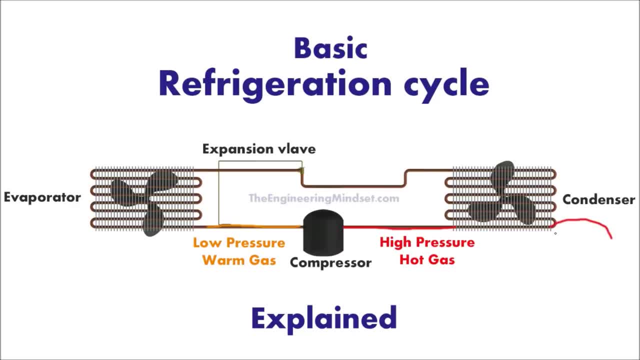 And that allows the heat to be ejected out of the condenser. Stage two happens at the condenser. The refrigerant enters the condenser from the compressor as a high-pressure hot gas. It passes through these coils here where it loses its temperature and cools down. 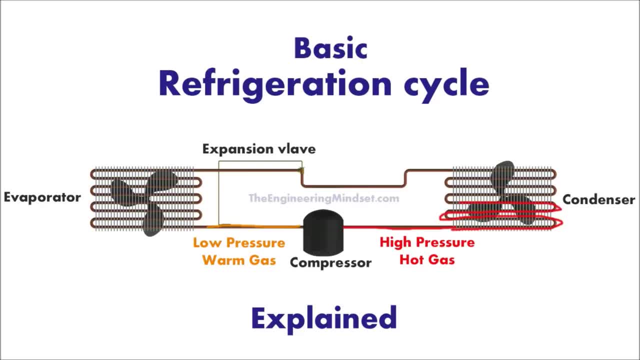 As it cools down, it begins to condense. It turns from a gas into a liquid, But it would be a warm liquid now, a regular temperature liquid, So that high-pressure liquid is going to be the condenser, Still at high pressure though. 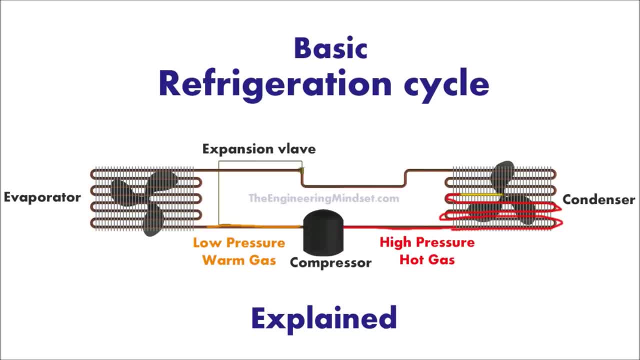 And just to indicate that I'll change its colour just to a yellow. So it's leaving the coil there. There we go. So that's going to leave as a high-pressure, regular temperature liquid. So this condenser coil. you've probably noticed that there's lines in between them. 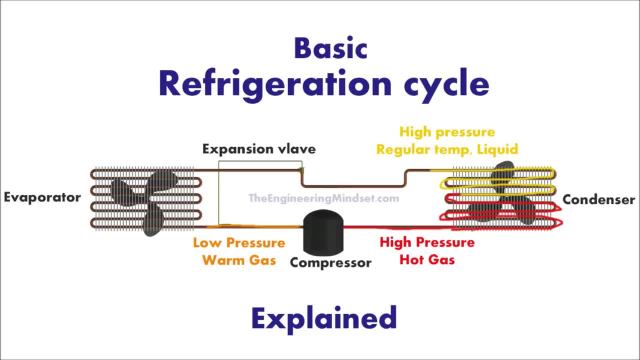 What's happening there is. these are: well, these are the fins of the condenser, And they're sheets of metal which touch the pipe, And that allows heat from the pipe to be carried away off into these fins in a method known as conduction. 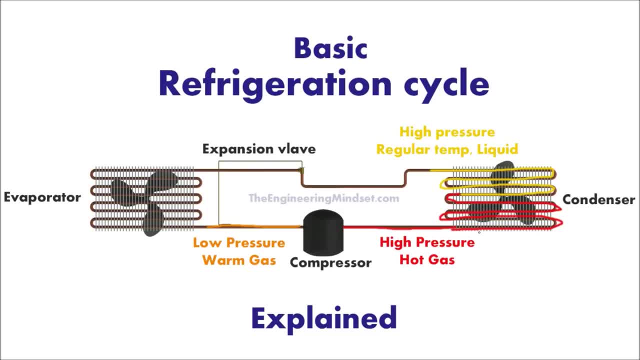 Behind the condenser coil is this fan And as that rotates it's picking up heat. It's picking up air- sorry, from the ambient air around the condenser pipe And that's forcing it through the coils And that air will then pick up the heat through these fins and also off of the pipe. 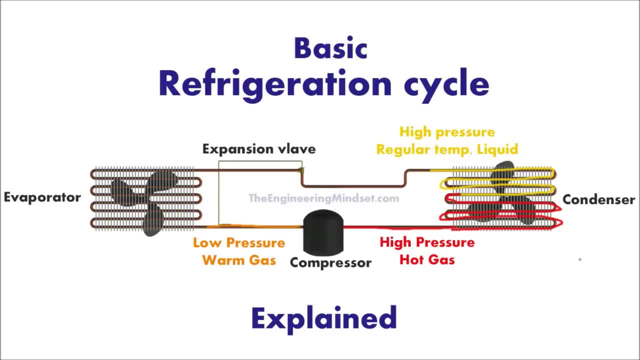 And it will carry it away and allow that heat from the system to be dumped, And that method is known as convection. Stage three happens at the expansion valve. The refrigerant enters from the condenser as a high-pressure, regular-temperature liquid. 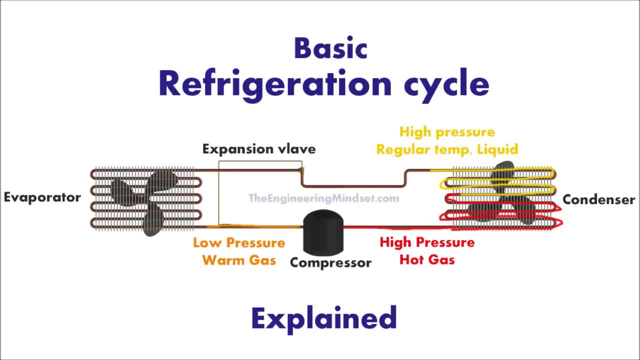 The valve regulates the flow of refrigerant around the system and into the evaporator. It does this using a diaphragm. Let's just draw on here, coming from the condenser to the expansion valve, So inside the valve body. here is a diaphragm. 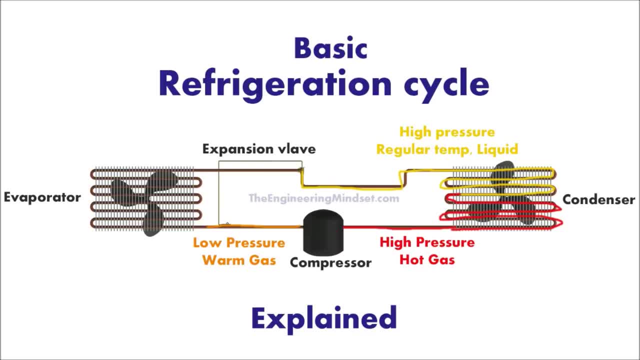 And the diaphragm is connected to a thermal bulb over here on the exit of the evaporator And it's connected by a capillary tube, that thin tube, that thin tube just there. The thermal bulb sits on the exit of the evaporator and inside there is another refrigerant. 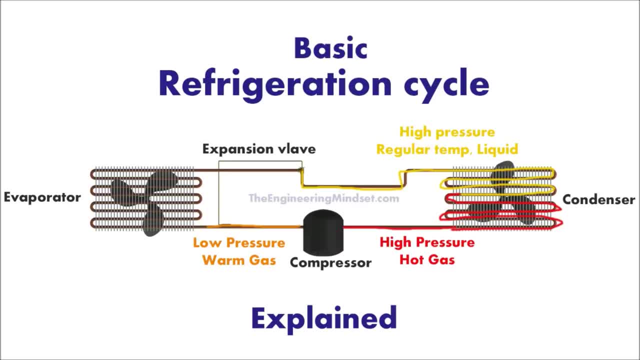 And that On the temperature of the refrigerant leaving the evaporator, the refrigerant inside the thermal bulb will expand or contract And this change in pressure in that capsule will travel along the capillary tube and that will move the diaphragm up and down. 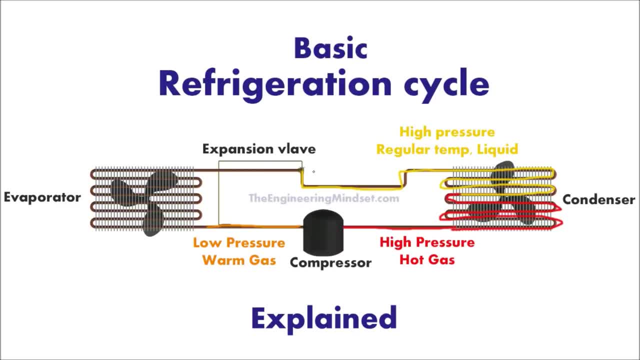 The up and down movement of the diaphragm will allow more or less refrigerant to pass through into the next stage. So because the valve restricts the flow, there will be less refrigerant on the exit, on this next pipe, here, the next section of pipe. there will be less refrigerant there. 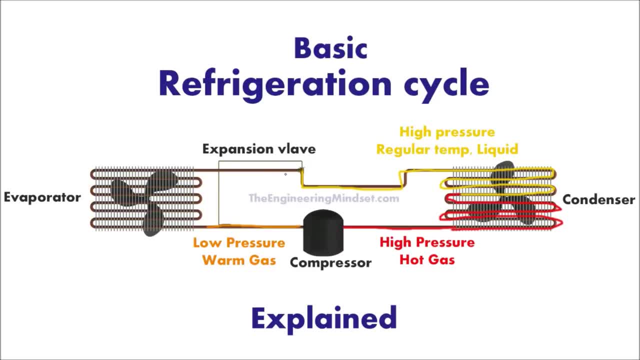 So there will be room for the refrigerant to expand. As it expands, the molecules within it move further apart and this drops the temperature and pressure of the refrigerant. So it leaves as a low pressure cold liquid And we'll draw that on there as well. 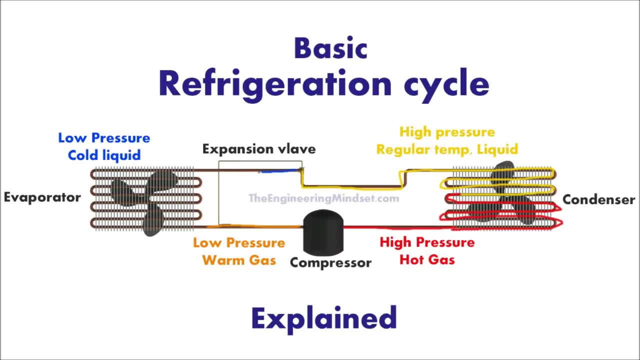 So as that leaves the valve and into the evaporator as a low pressure cold liquid. So stage four, which is the last stage in the refrigeration cycle, and this happens in, obviously, the evaporator- The refrigerant enters as a low pressure cold liquid. 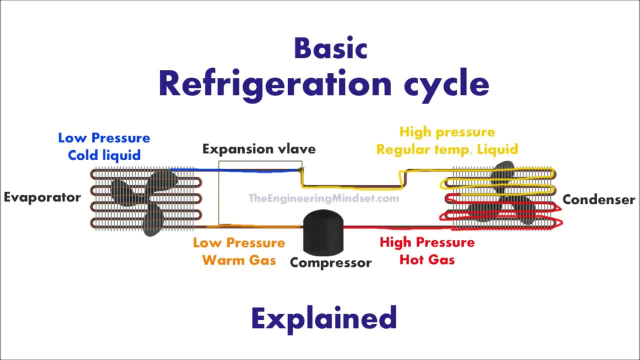